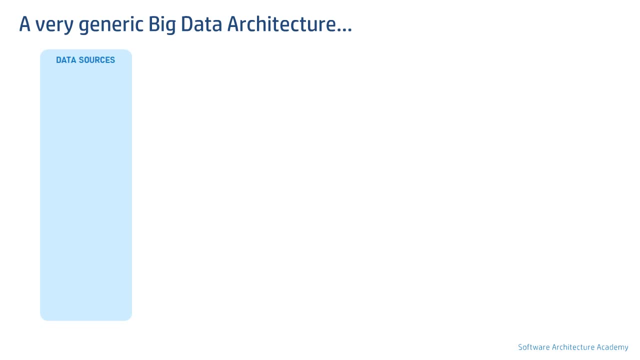 of big data is to ingest tons of data from variety of diverse sources. The data can be classified into structured, semi-structured and unstructured. So the structured sources can be our traditional systems like data warehouse, data mart, OLTP and ODS containing your organizational data. 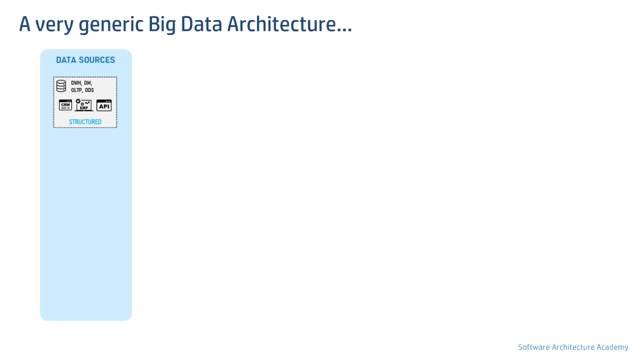 Further they can be CRM or ERP systems and, finally, exposed APIs. Now, what exactly falls under semi-structured and unstructured data can be debated. Organizations have their own classification mechanisms. We will be using our best judgment. How to Construct Substructured Data. 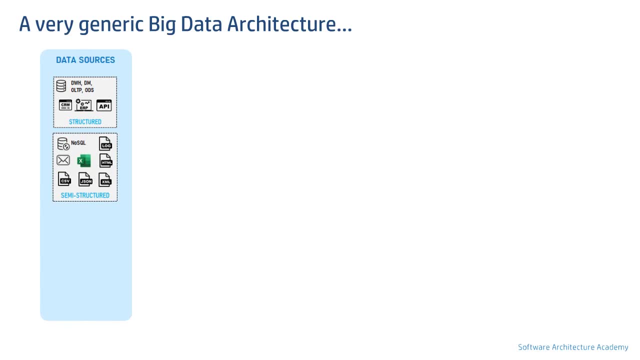 So what can constitute a semi-structured data? Well, no SQL database, to begin with. That make this different from structured data: Log Files. Next, Log files can be considered as semi-structured since there is some element of structure or patterns induced while logging from a code. 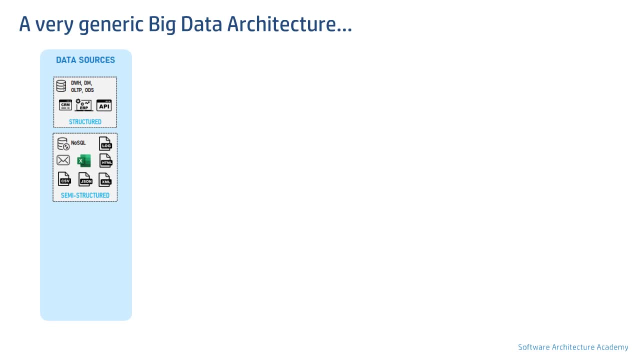 Email be another good example, since it has header subject to cc, bcc fields in structured format and email body in unstructured format. next, organizations use a lot of spreadsheets. a spreadsheet containing data without any accompanying schema or definition can be classified as a semi-structured data. and finally, html, csv, json and xml files are all examples of 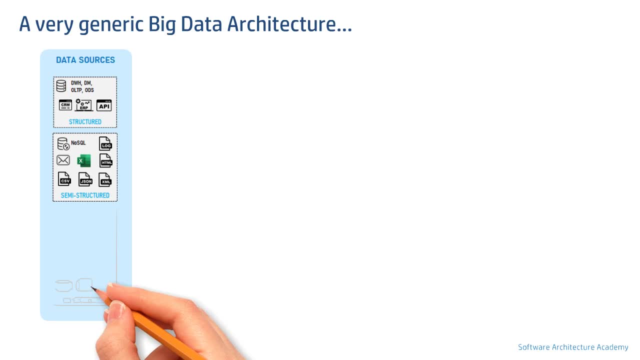 semi-structured data. moving on to unstructured data, it gets interesting here. multimedia groups like images, audio video can be our very first example. social media data streams can be our next. another good example of this category is messaging data like sms, whatsapp and chat, taking this a level further to explore full potential of big data. 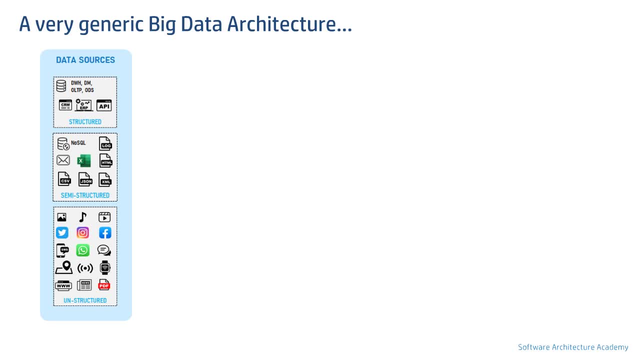 we can have gmail, gmail or maps, data, sensor data and data coming from smart devices like smart watches, etc. and finally, websites, web pages, online news articles and text in pdfs are all unstructured data. now that we have discussed sources, let's focus on the big data system side of things by covering 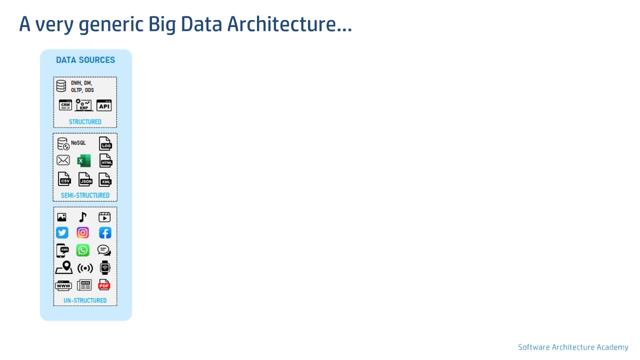 the different layers that are there. so how will we structure this conversation? we will cover this conversation in three parts. we will first discuss layers, then we will cover the layers that are in its components and finally, possible data flows. so let's first understand the different layers that are there in a big data architecture. 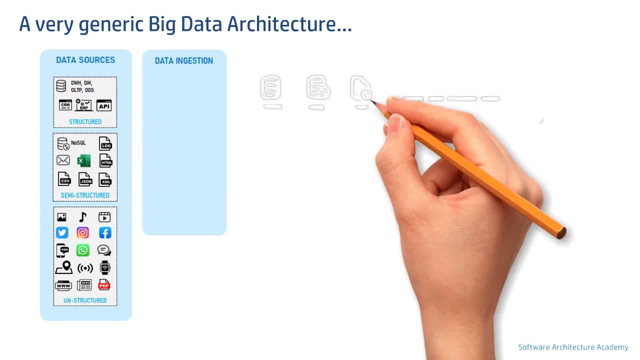 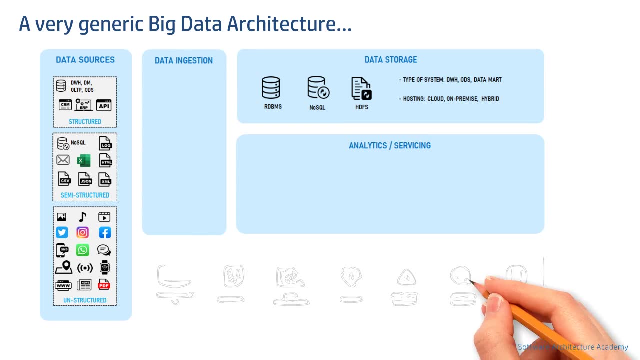 there can be ingestion layer, data storage layer, analytics layer, also known as servicing layers or simply service layer, data consumption layer and, finally, big data governance layer. please note that there are multiple ways to build a big data system, with or without all or some of these layers. in order to handle different them, maybe by discriminating different layers, i've here tried to. 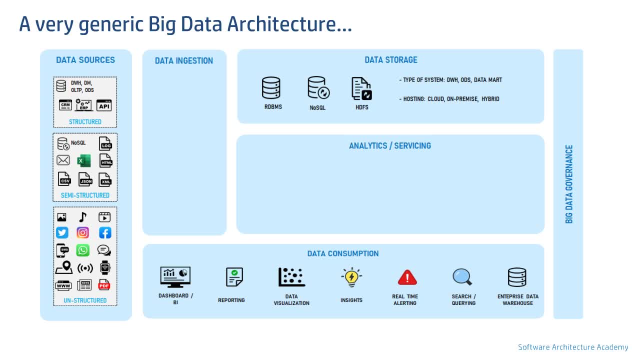 generalize and combine few layers for the sake of simplicity. since this is a generic reference architecture, focus here is at high level and on learning. now two things to note here. first, you must have seen a dedicated processing layer shown in some big data architecture diagrams. processing is basically moving data from one layer to another, hence the processing layers, namely batch. 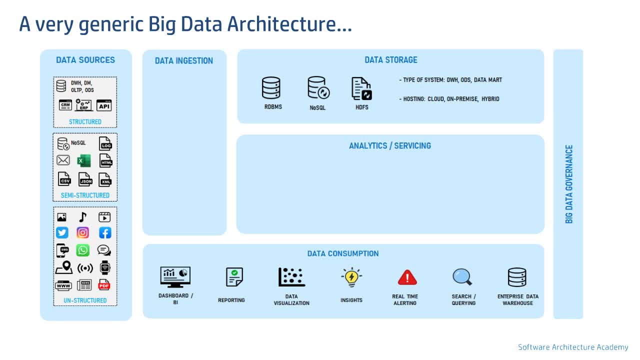 and real time would be over arcing these layers that you see. i will be showing more detail in the next few minutes, showing these type of processing in the later part of this video. Second, I have combined analytics and servicing layer by showing analytical processing and 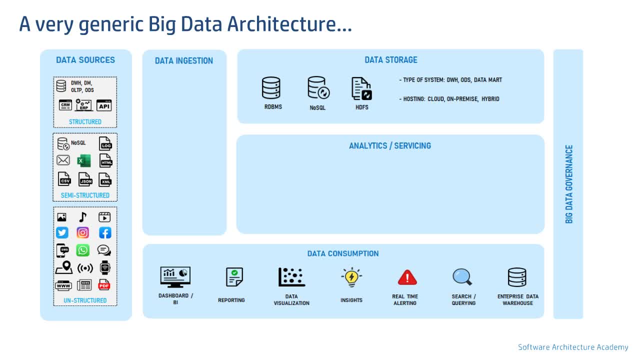 its pre-computed outputs into one. Also, all on the fly or in-memory activities will be shown with the help of arrows. Now, coming to a second part of the three-part conversation, let's discuss the components of these layers, starting with ingestion layer. 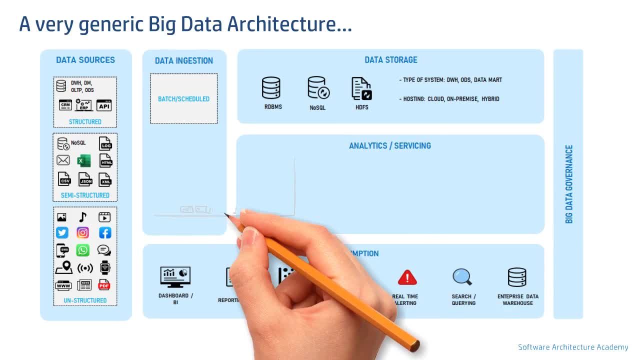 There can be a batch component and there can be a real-time or stream component, which is the true differentiator of a Bing data architecture from a data architecture Coming to storage layer. there can be traditional relational databases to store structured data and, yes, at times semi-structured data as well. 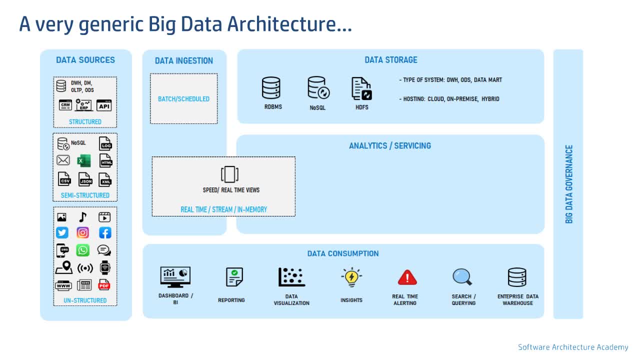 Then there can be one of many types of NoSQL databases to store structured, semi-structured and unstructured data, And finally we can have a Hadoop distributed file system, which is a fault-tolerant distributed file system. Next one is the analytics or serving layer. 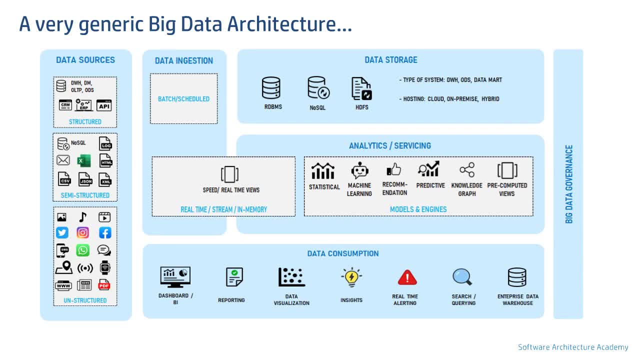 This is the layer where models and engines run and provide outputs to be utilized by a consumption layer, typically on-demand. It can have statistical and AI models. It can have recommendation engines, like those Amazon product recommendations or YouTube video recommendations. It can have a knowledge graph, which is widely used for link analysis and social media, and 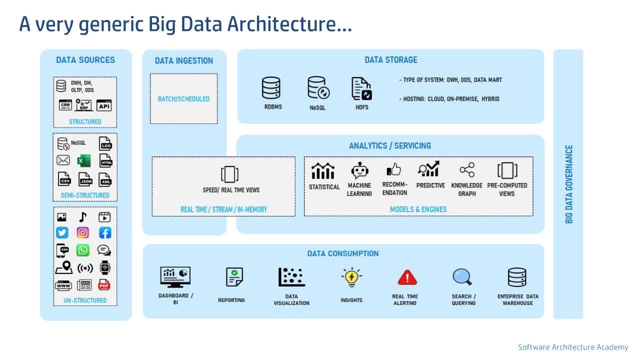 analytics And, finally, output of these models and engines, which are usually pre-computed views for user queries. Now, talking about data consumption layer, it can have a range of things that an end user or a target system needs. Most likely, these are BI dashboards, reporting, data visualization, insights generation, real-time. 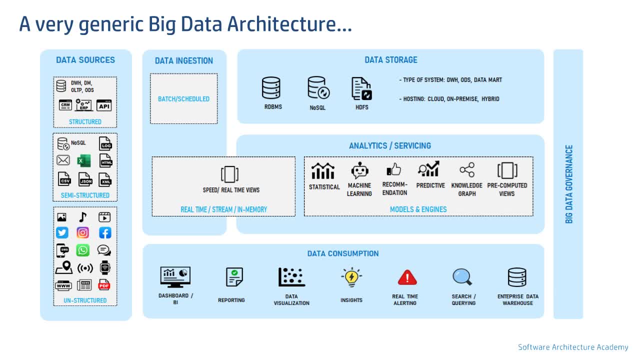 alerting, real-time searching and query capabilities And, finally, downstream systems. These are the systems that are usually used to do the most of the work, and these are the systems that are usually used to do the most of the work. And, finally, we have big data governance layer, which is used, as here, as an umbrella term. 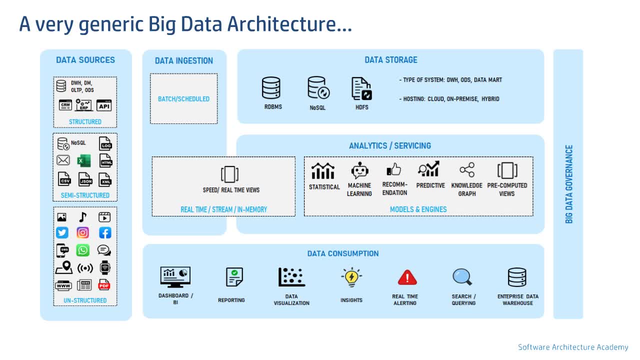 for data management activities like data auditing, data security, data quality controls, data catalog, metadata management, etc. Please note that a big data system has high chances to fail if big data governance is the most interesting one that is possible. data flows. 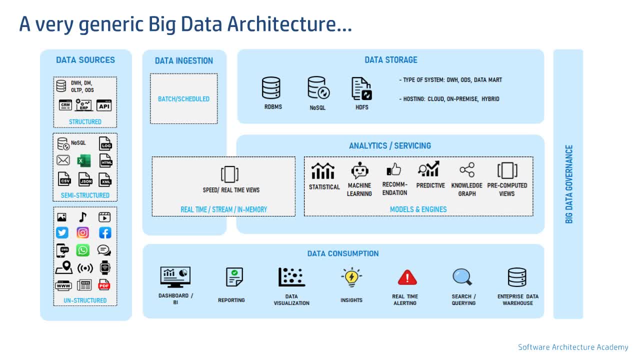 Okay, broadly, there could be two flows with variants. These flows are batch and real-time. Let's start with the batch side of things. A batch is scheduled, hence periodic, and it should write to a dedicated storage before any analytical activity can happen. 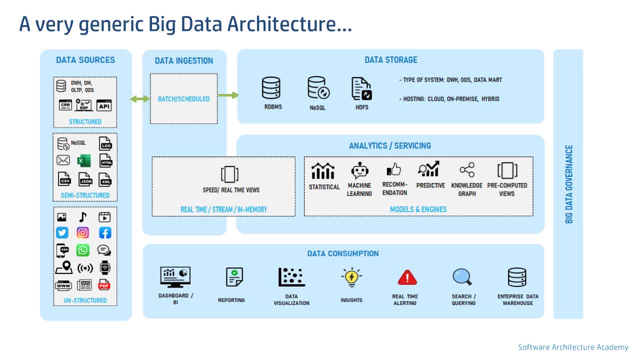 It's used for cases where historic data is of significance and where history data needs to be maintained. For push flow, The data is then sent to analytical layer, typically in a scheduled fashion, then processed and finally sent to downstream For pull flow triggered by a consumption layer. analytics layer picks up the required data. 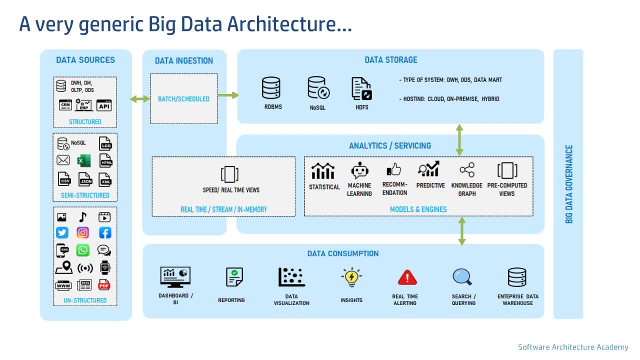 from storage layer processes and fulfills the request. Now let's talk about real-time or stream side of things, which makes this a big data architecture in truest of sense. The first flow here Here Is when a request is catered in real-time by in-memory processing with the help of computing.